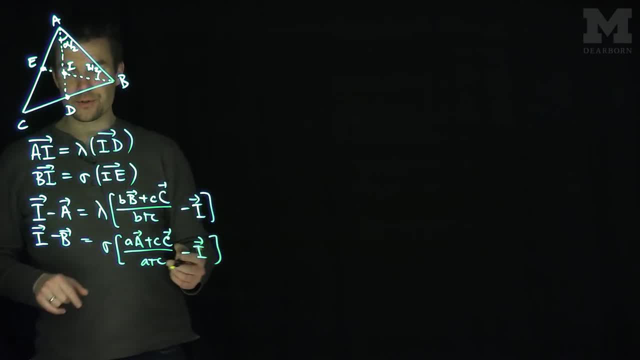 And so from these two relationships over here we get two different formulations of what I is going to be equal to. So this first equation here says that 1 plus lambda times- I is going to be lambda times- B, B plus C, C over B plus C and then plus A. 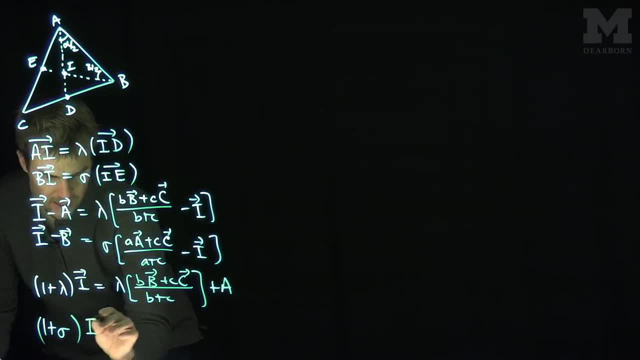 And then I have 1 plus sigma times, I is equal to sigma A, A plus C, C over A plus C. And then I have 1 plus sigma times, I is equal to sigma A, A plus C, C over A plus C and then plus B. 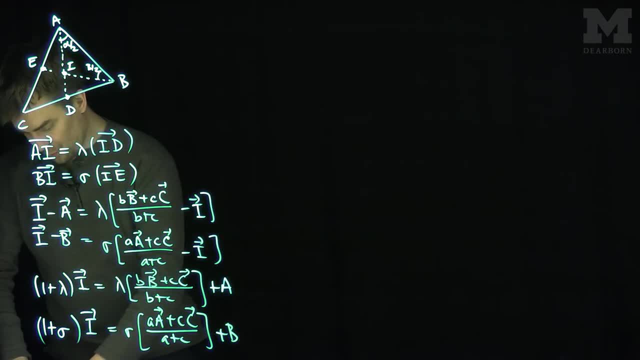 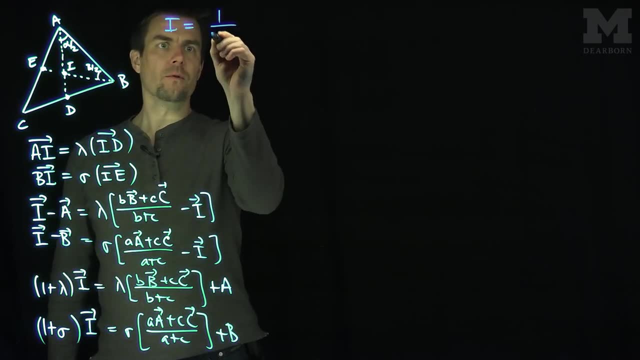 And so I get two different representations of I from these formulas. The first representation we get is this: We get that I is equal to. from the first equation is going to be a: 1 over 1 plus lambda times A, plus lambda over 1, plus lambda times B over B, plus C in the direction of B. 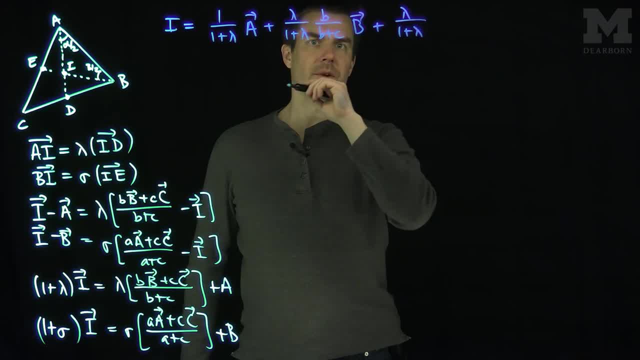 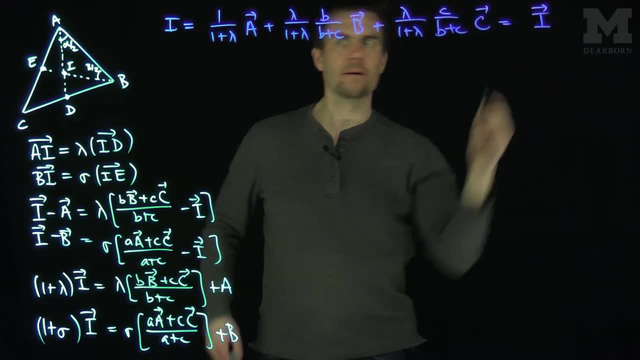 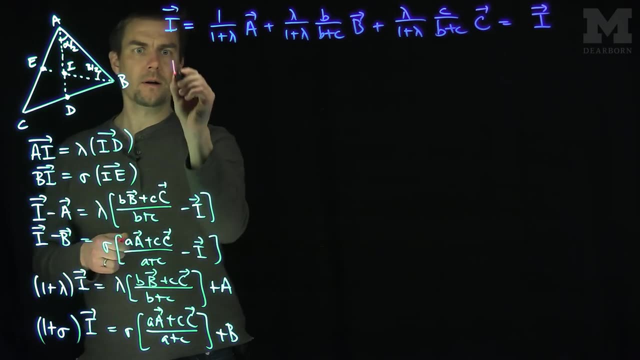 plus lambda over 1 plus lambda, and then C over B plus C in the direction of C. This is one representation of I, And we have another representation of I. I is also represented by this vector over here. I is going to be what? 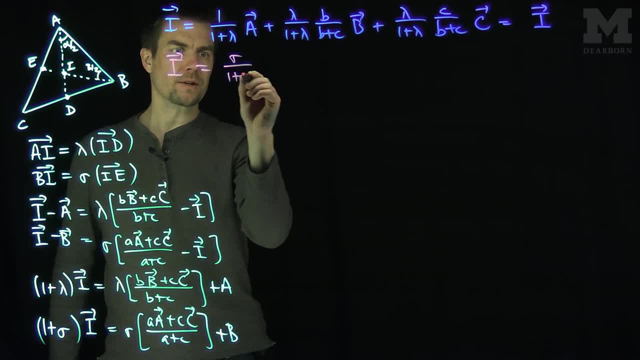 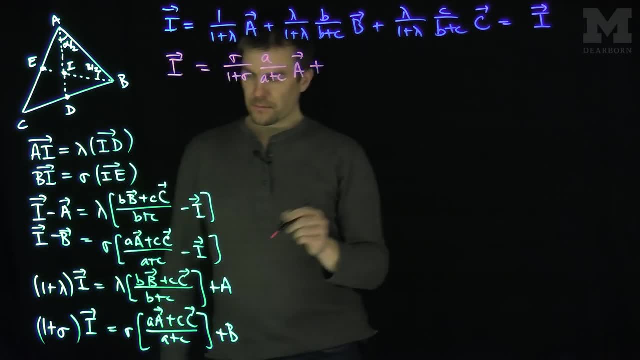 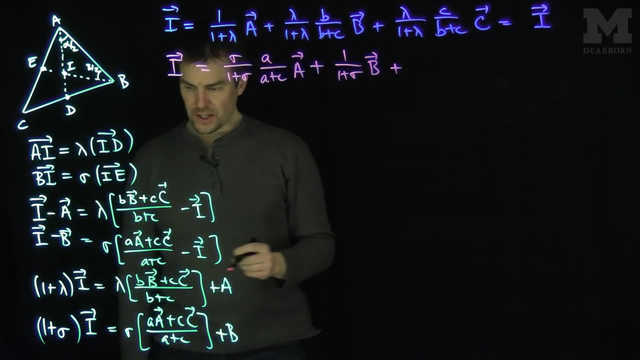 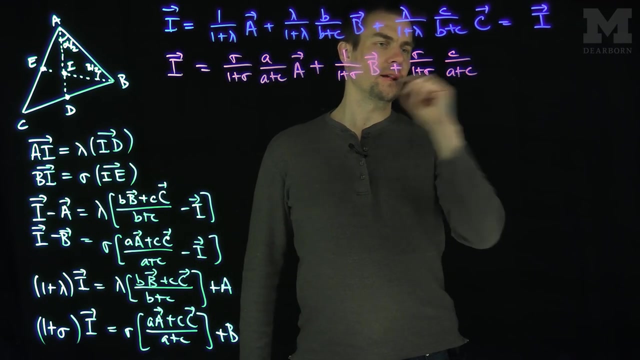 It is going to be sigma over 1 plus sigma, times A over A plus C, A plus 1 over over 1 plus sigma, B plus sigma over 1 plus sigma, sigma over 1 plus sigma, and then C over A plus C over A plus C. 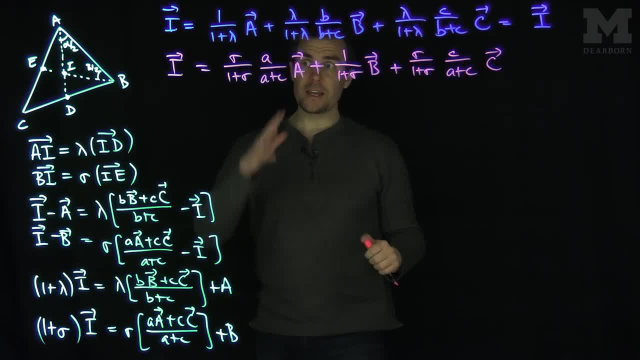 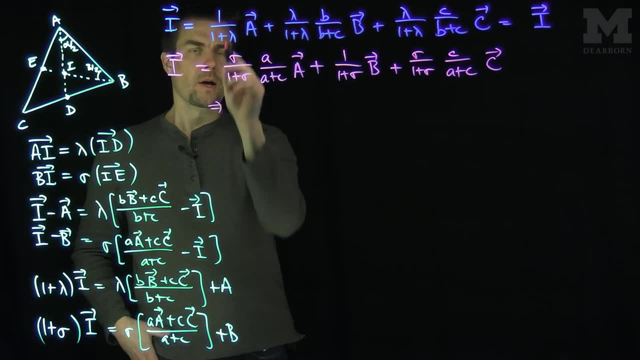 in the direction of C. So I have two representations of the in-center as a vector. Now I can equate coefficients. The first thing we can conclude from this is we can conclude from this that 1 over 1 plus lambda is equal to sigma over 1 plus sigma. 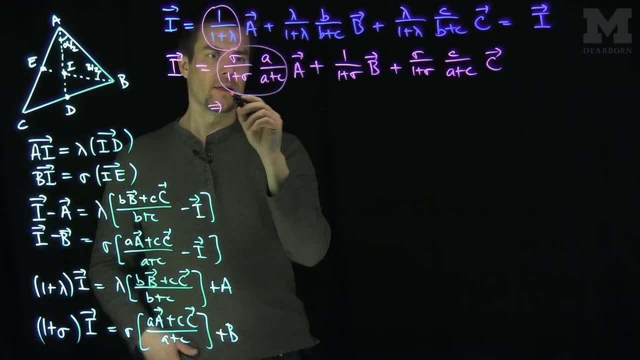 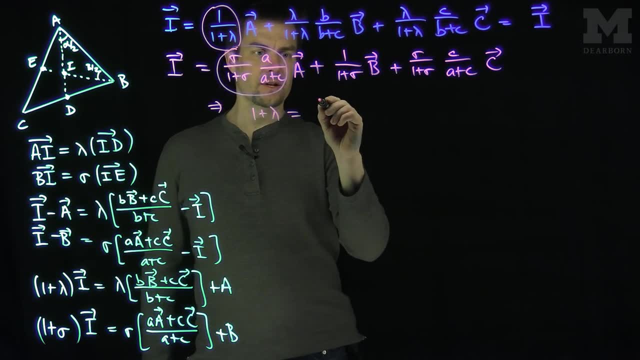 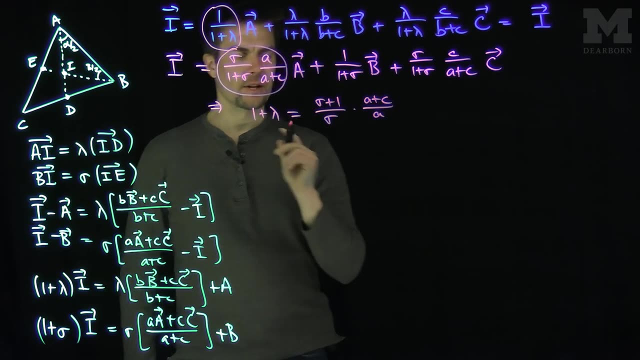 over a plus c. so from this I can conclude that, or I can just take the reciprocal of those relationships to and conclude from this that one plus lambda is the reciprocal of this. so that's going to be a Sigma plus one over Sigma, times a plus C over a. that's one equation we get. we can also compute. 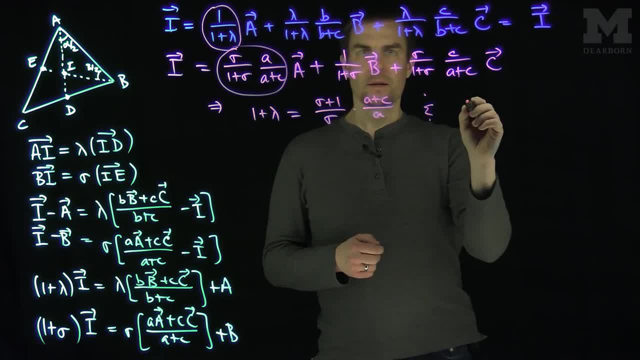 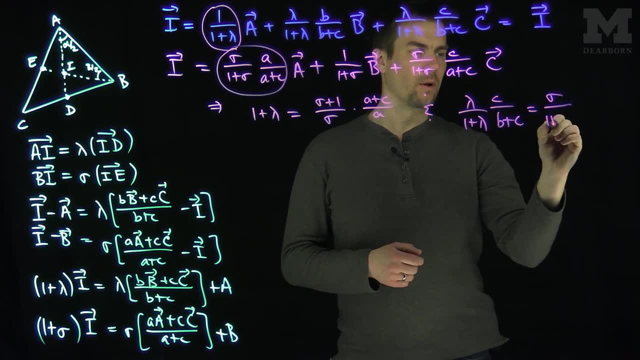 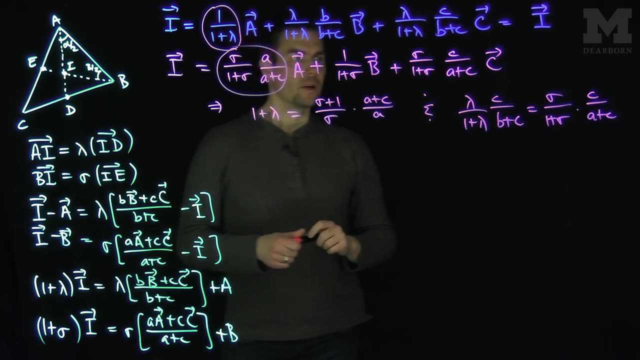 equate the coefficients of C. we also get that lambda over one plus lambda, C over B plus C is equal to Sigma over one plus Sigma times C over a plus C. that's good. so now we get from this- actually we can get a formula for lambda, because we know. 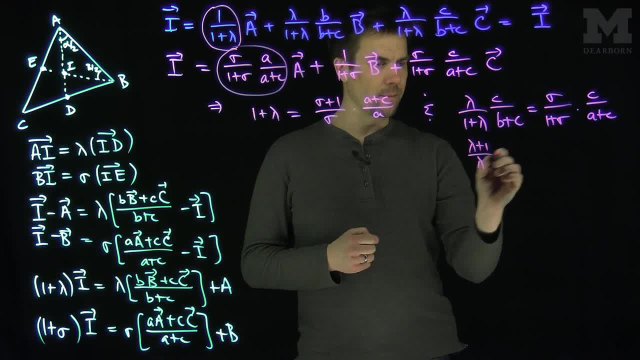 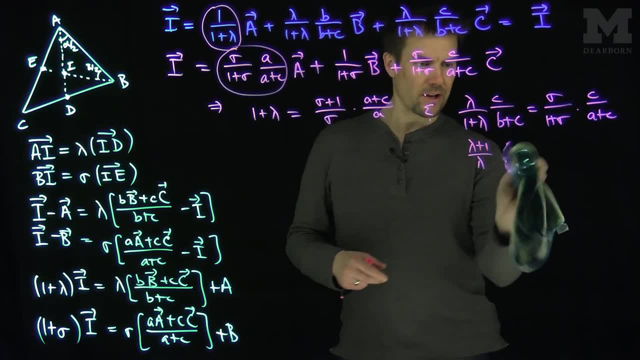 by taking the reciprocal of this, that one plus lambda over lambda, C over B plus C, the data reciprocal something, the reciprocal of both sides. so take the reciprocal of that as well. let's take the reciprocal of this. so the reciprocal this is this and the reciprocal this is B plus C over C. 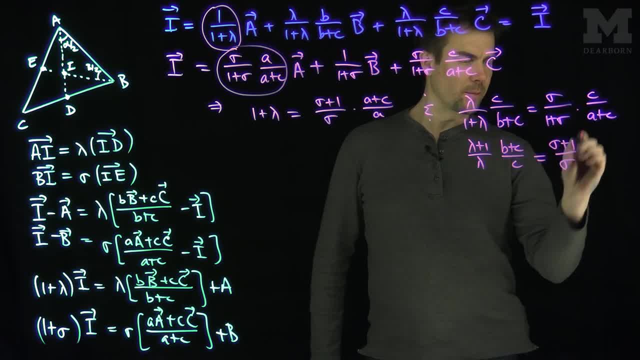 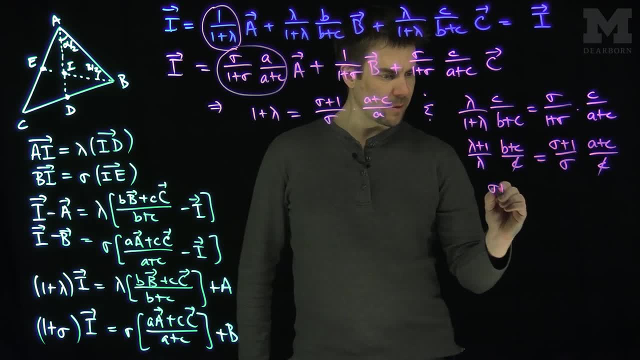 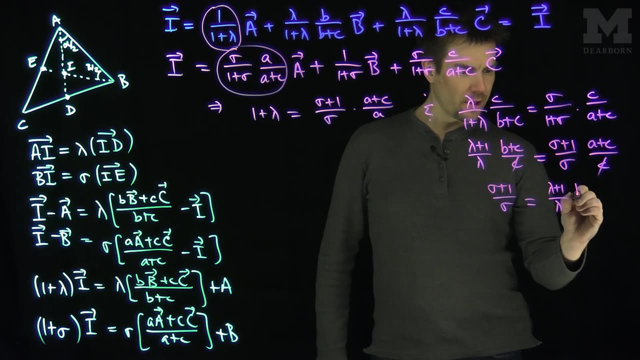 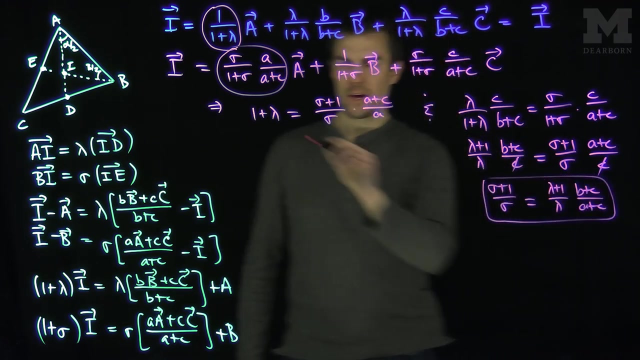 okay, is equal to Sigma plus one over Sigma. times a plus C over C. those C's are going to cancel on both sides equation and therefore we get that Sigma plus one over Sigma is going to be equal to lambda plus one over lambda, and then B plus C over a plus C. so that's my formula for Sigma plus one over Sigma. I. 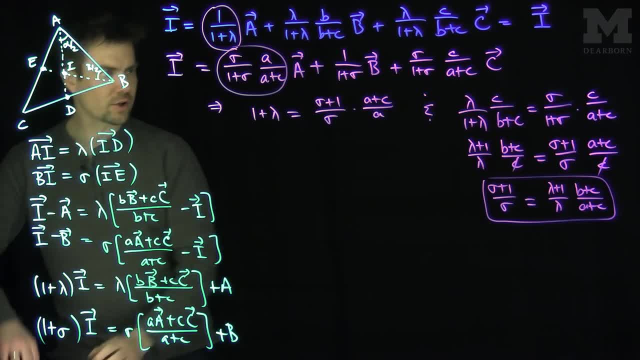 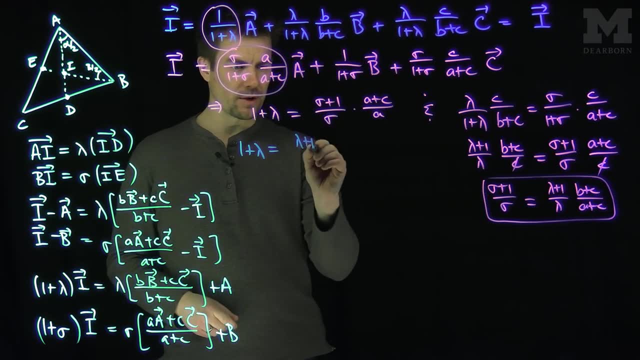 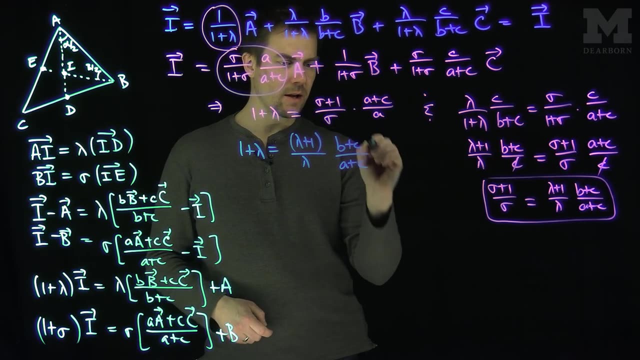 can fill it into this equation over here. let's do that. so if we do so, what we get we'll get one plus lambda. one plus lambda is equal to Sigma plus one over Sigma, which is lambda plus one over lambda times, B plus C over a plus C times. what times? 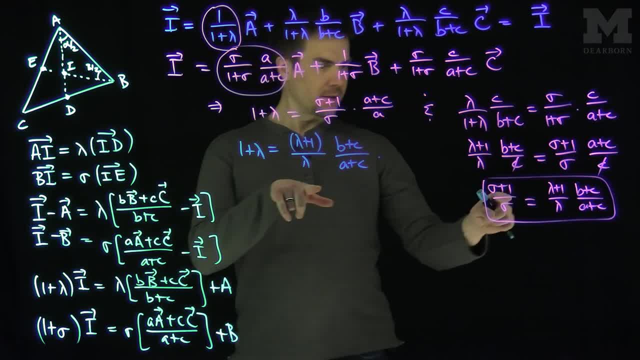 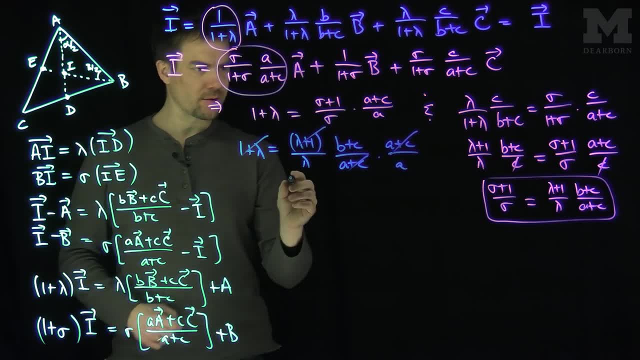 times. that's my sigma plus one over Sigma, and I have an a plus C over a. the the a plus C's will cancel the lambda plus one will cancel, and then I have my, and I'll be able to conclude from this that one over lambda is equal to. 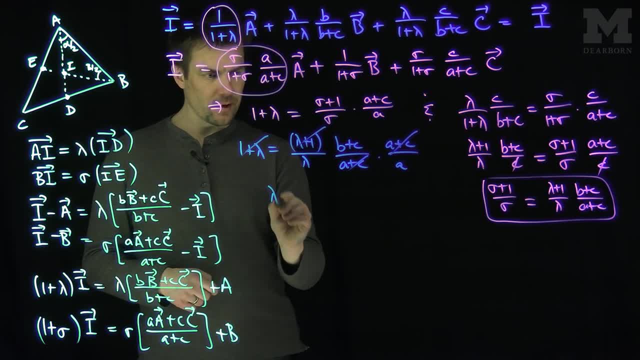 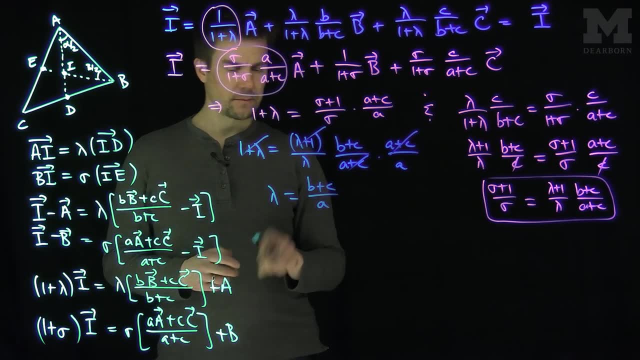 one over lambda times b plus c over a is equal to one, so lambda is equal to b plus c over a. So if I do one plus lambda, so one plus lambda, therefore, is going to be what? One plus lambda is going to be a plus b plus c over a. 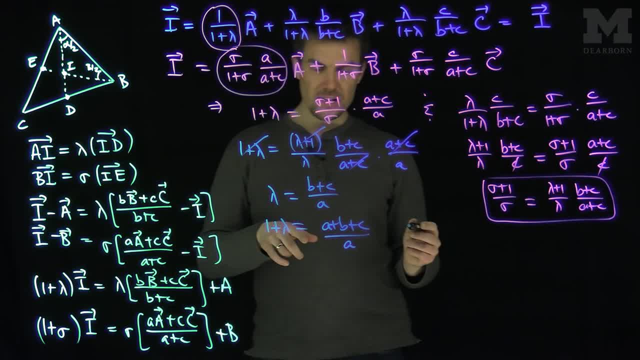 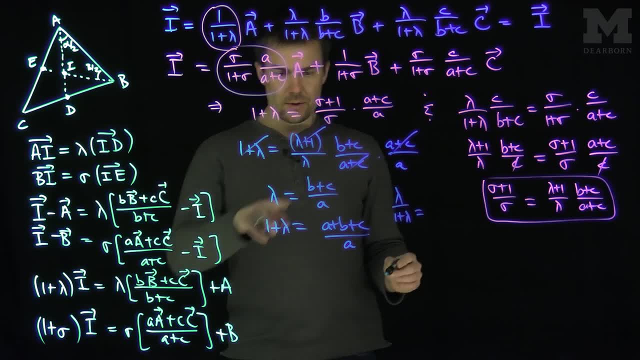 So we're in great position now, because let's do one final step. So the final step is to say what is lambda over one plus lambda. Lambda over one plus lambda is going to be this over this, so that's going to be b plus c, b plus c.